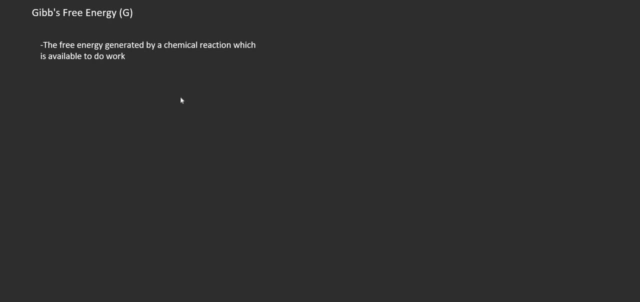 this might be of interest to you, Because when you think about the molecule ATP, adenosine triphosphate, we often hear in biology, whether in microbiology or other biologies, that adenosine triphosphate is used by our bodies, by our cells, for energy. 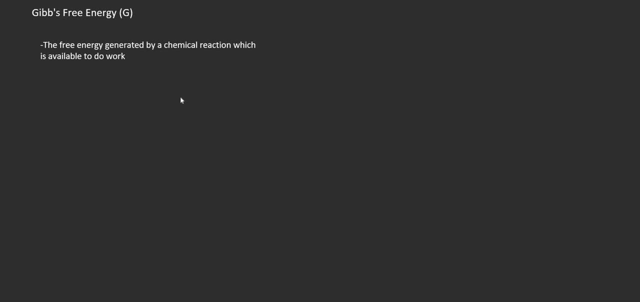 It's produced to use as energy throughout our body. But where does the energy from ATP come from? We know ATP is involved with energy somehow. Well, it just so happens that it's directly related to Gibbs free energy, The hydrolysis of the ATP molecule. 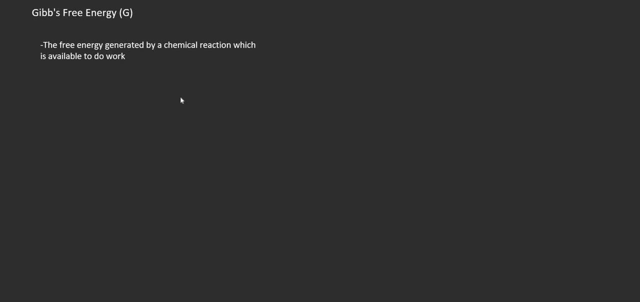 involves giving off of free energy. When you split apart ATP, you generate free energy through that reaction, And that energy that's produced from that reaction is what's used as energy in our bodies. So this is a little application for you. 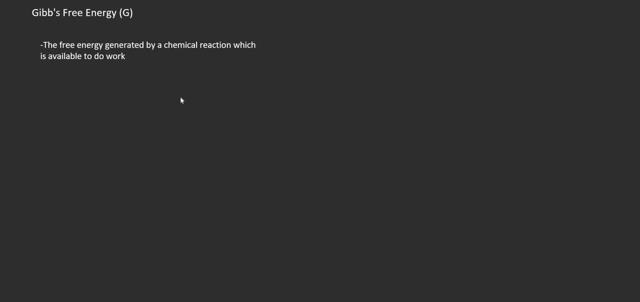 So delta G is definitely important stuff, But we'll be looking at it specifically from the chemistry side of things, And so, to use numbers with delta G, you can, of course, find values for delta G in tables that have been compiled and tabulated. 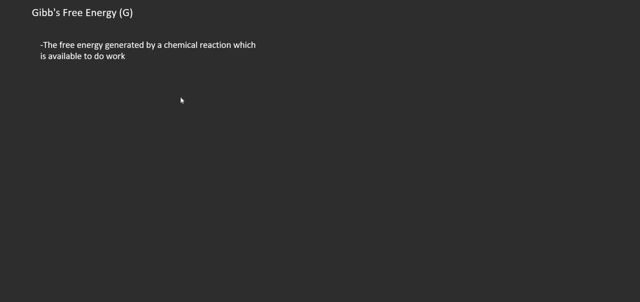 And you can calculate delta G for a reaction, the same old-fashioned way that we did for enthalpy and for entropy, Where you can look up values in a table and you can take the sum of the products minus the sum of the reactants. 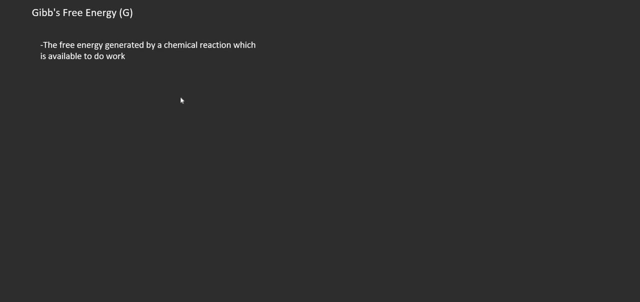 and that will give you your delta G, Your delta G value for your reaction. But delta G also can be calculated using a unified equation of thermodynamics, Where this equation will unify our three main state functions and temperature, So that unified equation is going to look like this: 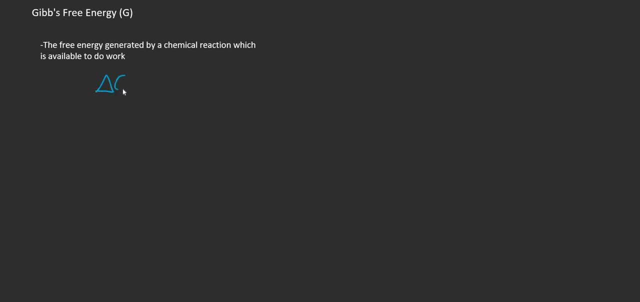 Where we have delta G being equal to delta H, minus temperature times delta S, And so, as you can see, this equation unifies. It gives free energy, enthalpy and entropy, As well as bringing in temperature. 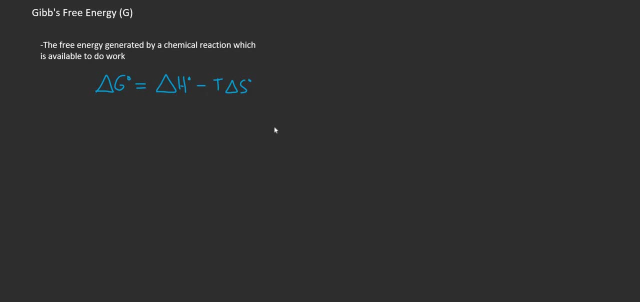 And this equation is useful when we have a constant temperature And we'll see that we use the value of delta G as a way to judge spontaneity of a reaction. So we could use a combination of enthalpy and entropy to judge the spontaneity of a reaction. 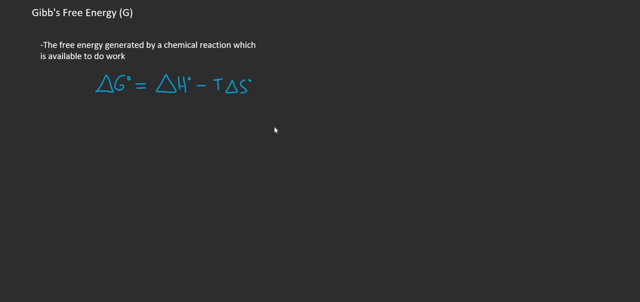 But it depended on whether you have high temperature or low temperature, whether your temperature is equal, whatever, But delta G, it sort of has the final say on spontaneity. When your delta G is negative, your reaction is spontaneous. 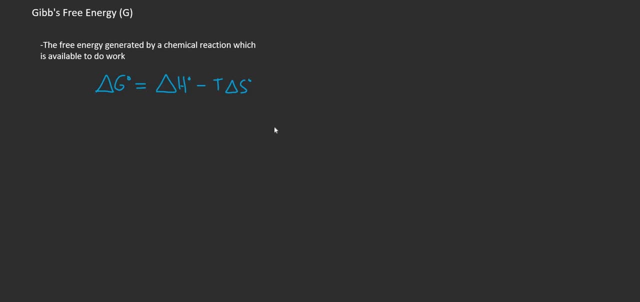 When your delta G is greater than zero, when it's positive, it's non-spontaneous, And when delta G is equal to zero, we have a situation of equilibrium. So delta G sort of has the final say when it comes to thermodynamics. 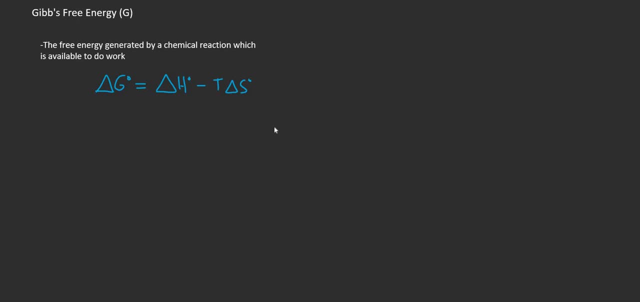 Which is why I like it so much, And this unified equation of Gibbs free energy is my favorite equation in all of chemistry. It is simply beautiful how it ties everything together. So what we can do now is we can look at calculating the standard delta G, delta G prime. 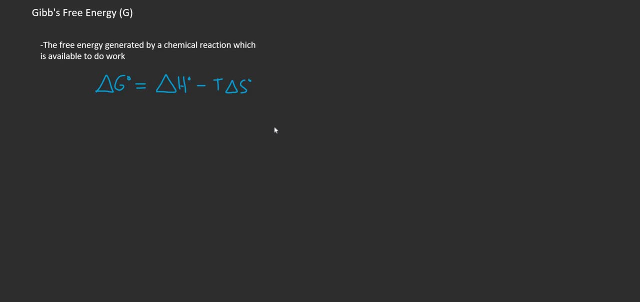 which is taken at standard conditions And we can look at how we can calculate for a particular reaction. So what we'll do is we'll take the reaction we looked at in the previous video, which was for entropy. So in the previous video we dealt with calculating the entropy. 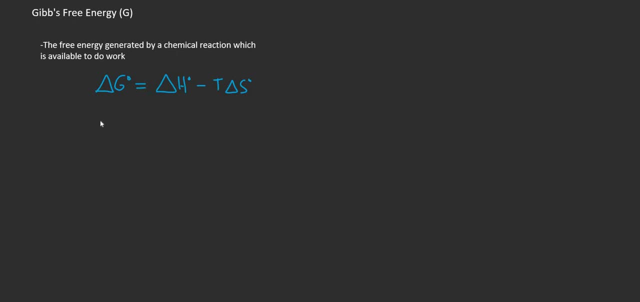 of the reaction And we're going to be looking at this reaction. So we'll have the reaction: 2SO3- gas forming oxygen, plus 2 sulfur dioxides, And, if you remember, in the previous video we calculated the change in entropy for this reaction. 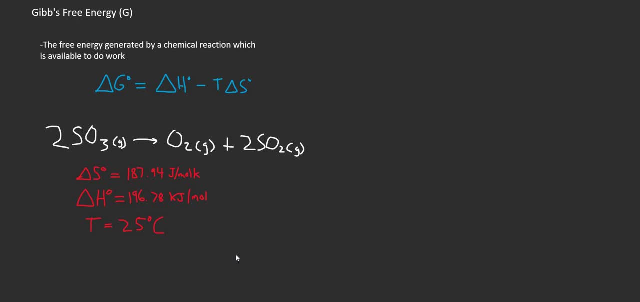 which is shown below as 187.94 joules- 187.94 joules per mole kelvin- And off-screen, sort of by magic. I calculated the delta H for this reaction using figures I looked up on an online table. 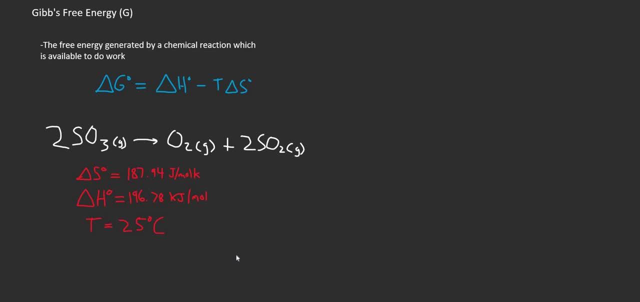 And so if you're a little squirrely on entropy and how to calculate that, I recommend going back and looking at the video on enthalpy And how to calculate enthalpy of a reaction. But it's literally the same way we calculated the entropy. 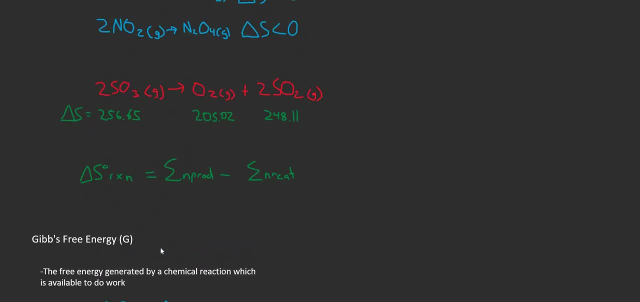 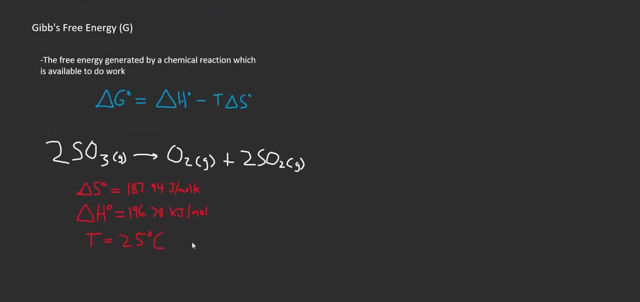 And so, and then our temperature. so we're going to do this at room temperature, which is sorry about that- .25 degrees C, But we're going to need to do some changes here, So our units need to match. 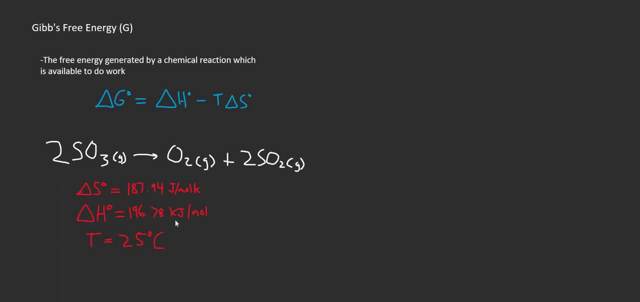 We need to have some units that work for us. So if you'll notice that the entropy is in joules, We need that to be in kilojoules Because we want to represent our delta G value in kilojoules. 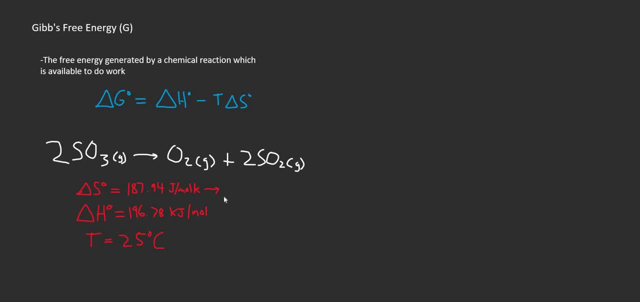 So these joules need to be changed into kilojoules. So, if you remember, there are a thousand joules in one kilojoule. So we'll divide this number by a thousand And you'll get. 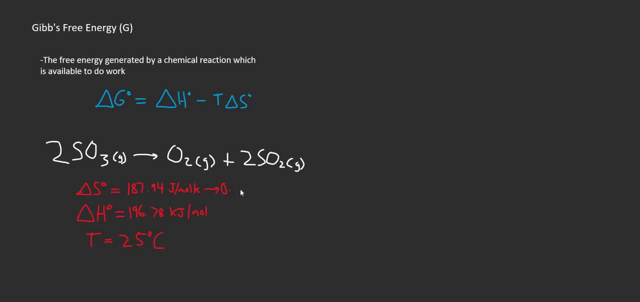 .0.18794.. kilojoules per mole kelvin And that'll get you that. Then our temperature. So our temperature needs to be in kelvin, so it can cancel this k up here. We don't want this k in our final units. 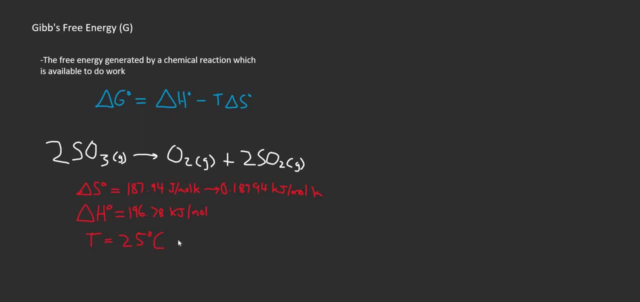 So we need to convert our temperature into kelvin in order to cancel that k out. So we'll simply add 273 to this number And it will be 298k, And this is something I would probably just keep in mind anyway. 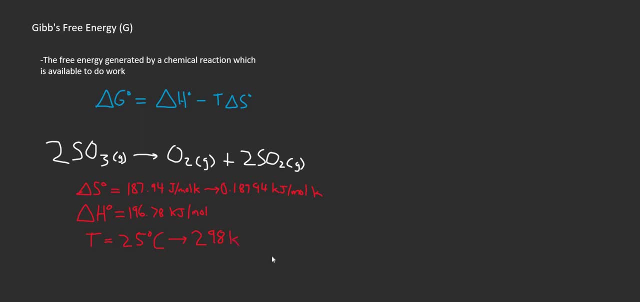 It's pretty easy to remember. Whenever you see 25 degrees C, I would immediately write down next to it 298k, Because 298k is what we consider to be SI units for standard temperature. So I would always try to keep that in mind. 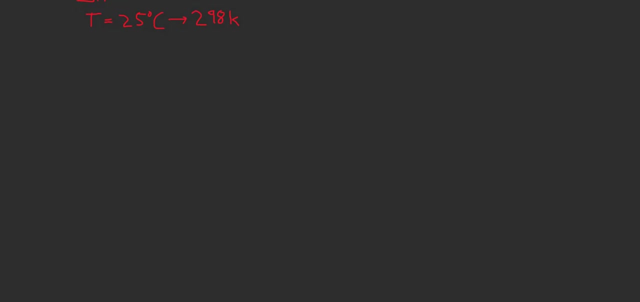 So now, if we want to calculate delta G using these numbers, what we can then do is start plugging things into our unified equation up here. So what we're after is delta G And so. 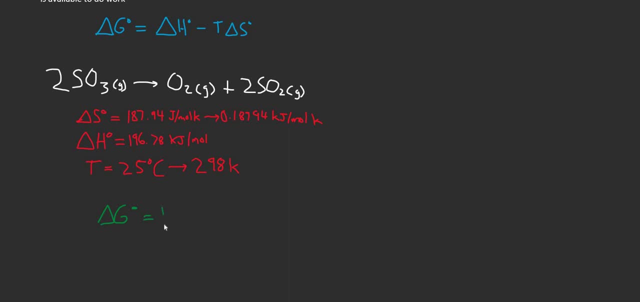 we'll start plugging in. So our delta H is .196.78.. And we'll subtract temperature, which is 298.. times delta S, entropy, which in kilojoules. 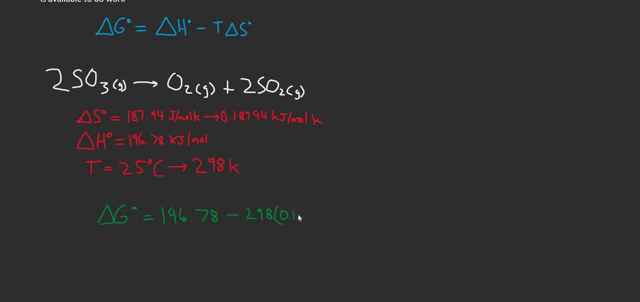 and it's very important that you convert this into kilojoules. I cannot stress that enough. Okay, And if you want, you can go ahead and do this calculation off camera on your calculator. You should end up with as your answer. 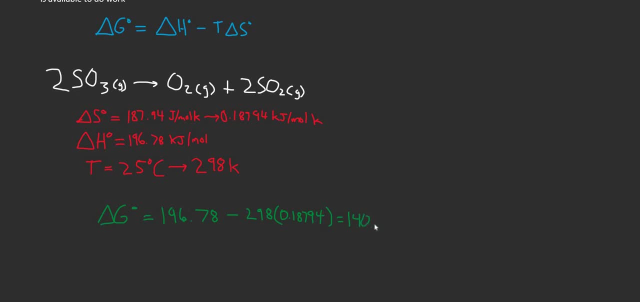 is 140.. point .77.. And don't forget your units, kilojoules per mole. So this will be your final answer. So how do we judge this? So you'll notice that our delta G